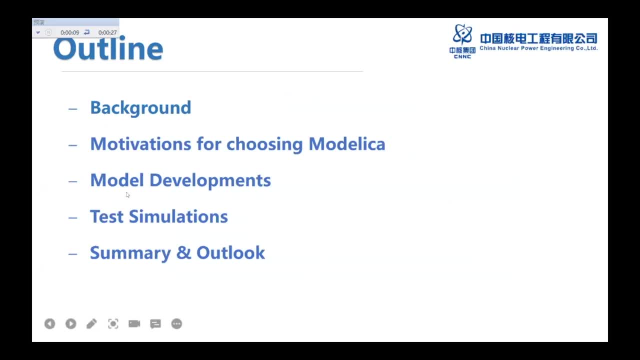 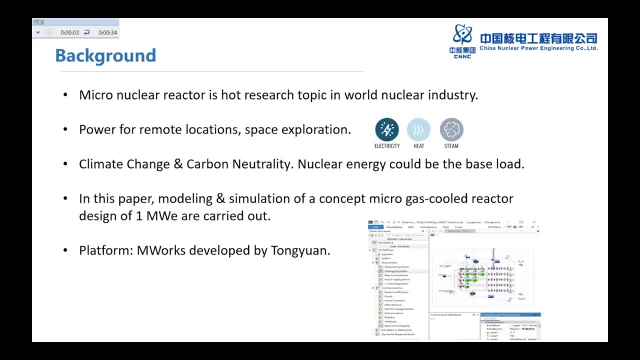 motivation why we choose Modelica, model developments, test simulation and the summary and outlook. First background: Nowadays the micro nuclear reactor is a hot research topic in world nuclear industry and this has wide applications such as supplying electricity or heat or steam in remote area with the pool traffic, for example island, and also because it's high energy density. 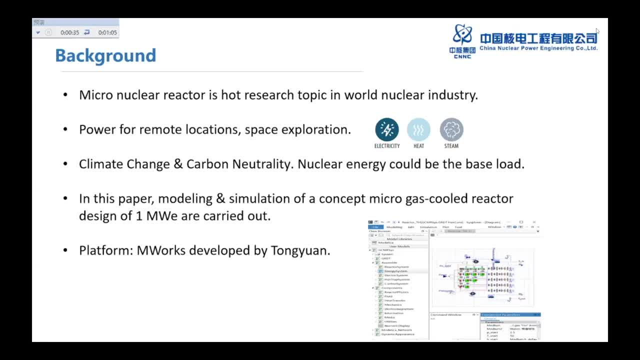 it can provide energy in the space exploration. And another important issue is the climate change and carbon neutrality. Now it's a global consensus because the nuclear energy is much more stable than other forces. In this paper, I will talk about the modeling and simulation of a concept design. Yes, this design is 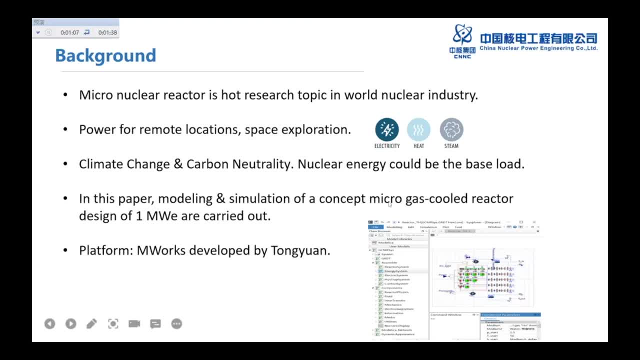 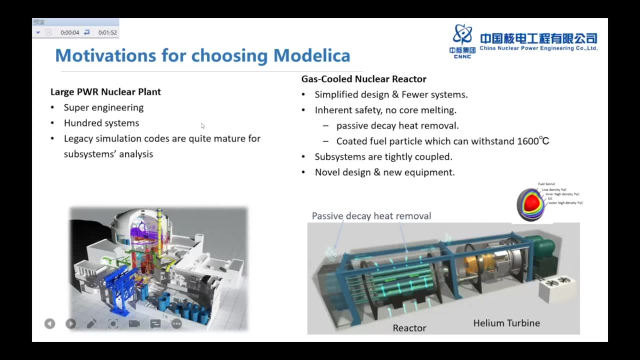 at a very preliminary stage. We use a gas-cooled micro reactor and the simulation platform is M-Works, which is developed by Suzhou Tongyuan company, a Chinese company. Here I want to discuss about why choosing the Modelica, Because let's look at the 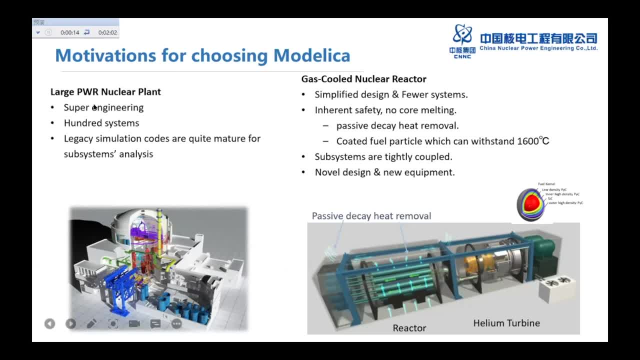 large nuclear plant first, and its super engineering consists of usually 100 systems and a lot of legacy. simulation codes are quite major for the subsystem design, But most of this absorbed in nearly a hundred systems. so let's take an example. one is this model here from REAL Auction. This model is of the Propentherm��, youngest model, Nerd into properties, and is designed in the 600th Beloved project. the first one is this one in Europe, The second one is from F Apartments. This model has been developed in recently as part ofALP and Mass Iなん proximity. Out of these you see, this model is in continuation of the 40th 200 modernalen de model In the 300th tengenge montagne, of the first local model here in Algeria. So there are thấy. 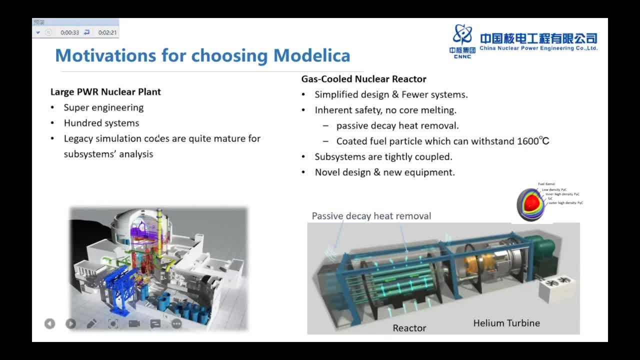 most of these legacy simulation codes were developed maybe 20 years ago, 30 years ago, So these codes usually simulate one subsystem or a few phenomenons. But for novel designs, such as this gas-cooled nuclear micro-reactor, we have some novel designs and we have new equipment. 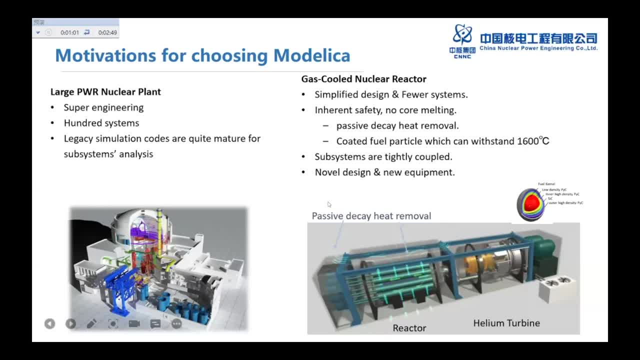 So we need to develop some new models, and the legacy simulation code cannot be well suited for this kind of analysis. And this gas-cooled nuclear reactor we developed is a very simplified design. It has fewer systems and it has good inherent safety performance. The core melting cannot happen because the safety is guaranteed by several. 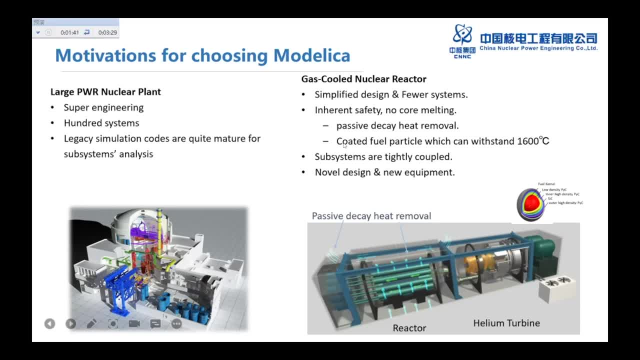 features. For example, we use better and stronger coated fuel particles like this, And this fuel particle can withstand a very high temperature and will not damage, And because of the total nuclear power, heat power is much smaller than the large one, So the 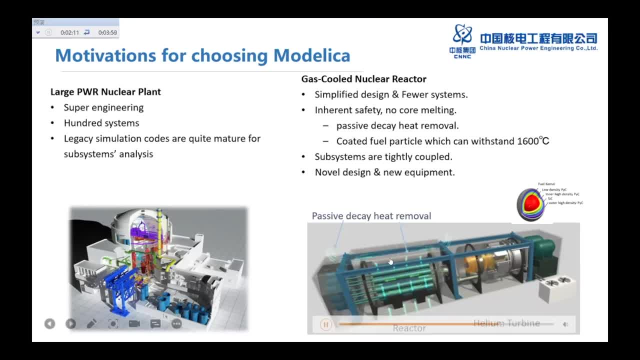 decay heat of the power can be removed passively by the air convection through the reactor pressure vessel wall And also because it has an integrated design. all these subsystem are tightly coupled, so they need to better simulate this coupling issue and the multi-disciplinary simulation must be performed so that we choose Modellica. 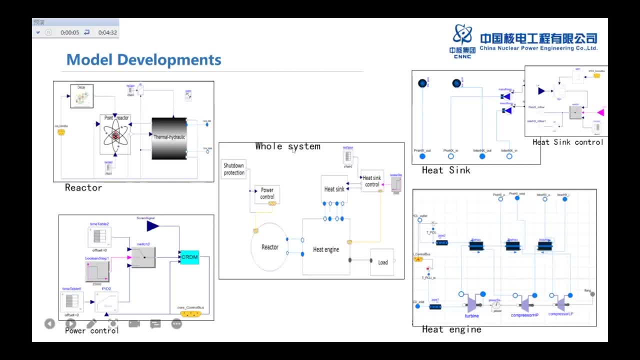 Here is the Modellica model we developed. It includes the reactors Hemi-S옵y-Heteronics. we use helium as the coolant and the helium heated by the reactor and then enters into the heat engine. The heat engine uses the Bruton cycle helium engine and then the heat. 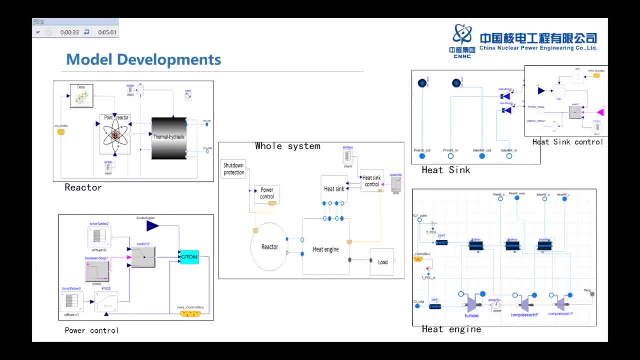 is converted to the mechanical power and then the mechanical power will be converted to the electricity power. electrical power by the generator and also the heat sink connected to the heat engine and provide provides the coolant water of the heat engine. Also, some control systems, such as like the power control system or shutdown protection system, are 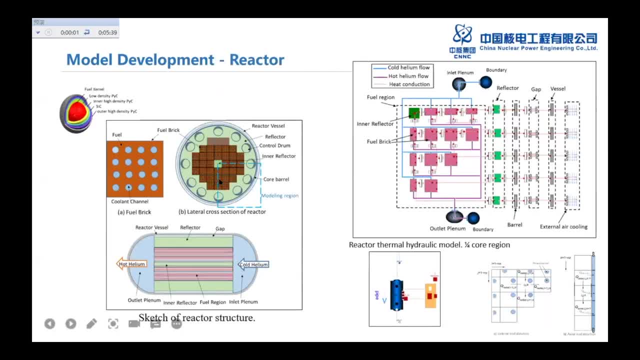 simply modeled. in this model- Now it's a vector sketch- you can see The reactor core is composed of 36 fuel bricks, these square bricks, and, and here, inner reflector assembly. so under the core it is the green color, green color which is graphite, and then a 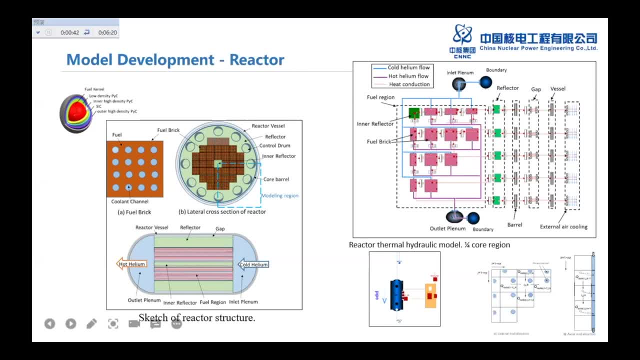 few Particle. the, your remaining fuel is dispersed in this orange solid region And mixed the graphite and This green. this holes are the flow channel, the helium can flow inside it And, due to the cyanometry, so they model the one quarter of the region in this thermohydraulic. 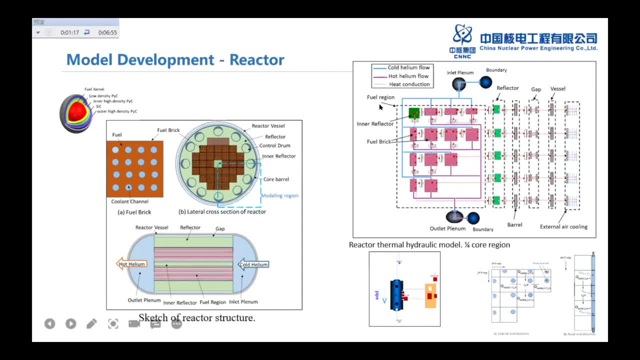 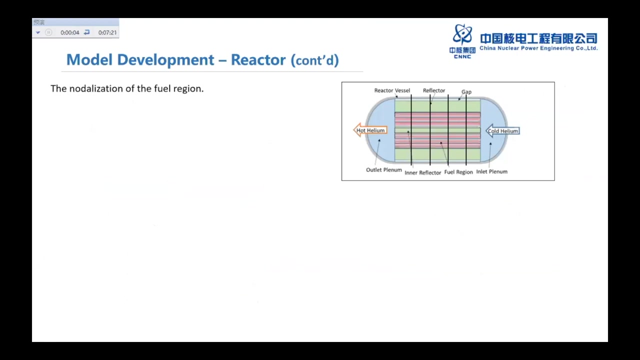 modeling and each reflector fuel bricksños and govern what is called uploaded by steels and the vassal vector pressure vessel and the external cooling and also the plenum, the inlet and outlet are here. This is the nodalization of the fuel region. there are 13 lateral nodes, each represent a brick. 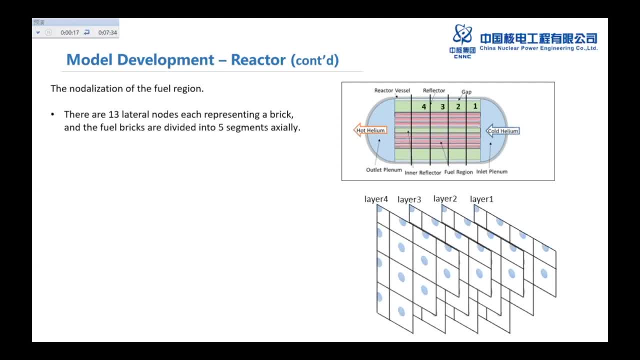 and the fuel brick are divided into five segments anxiously. therefore, there are 65 blocks of. each contains a solid fuel block and a flow segment. we use a parallel uh flow channel uh to to just one one flow uh flow pipe, but it's a represented the parallel. 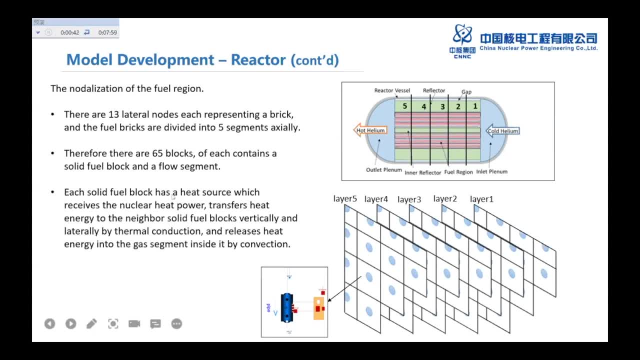 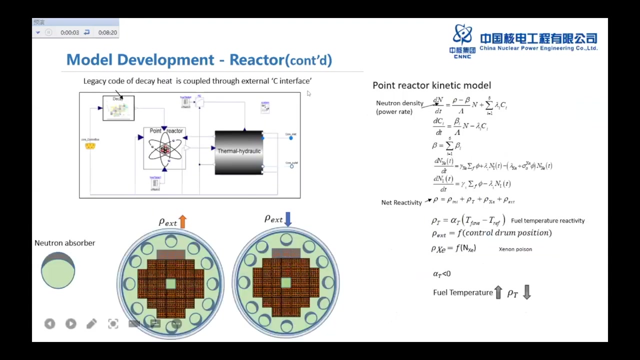 flow channel channels and each solid fuel brick have a heat source which receives nuclear heat power and the heat conduction uh, at the of the three-dimensional uh, in fact uh, uh, uh model that he also here this slice, gave a simple instruction about the reactor physics. they use the point reactor kinetic model here. 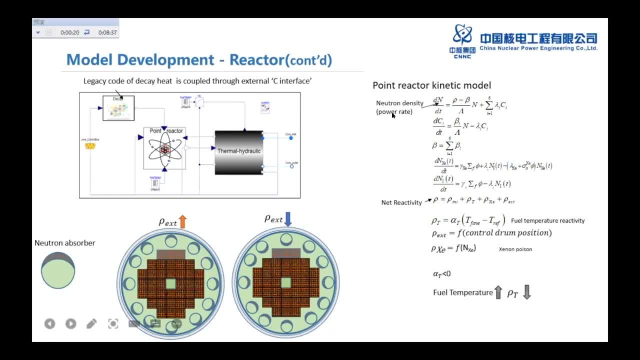 as you can see, the the nuclear heat power rate and is related to the reactivity role. if the uh- this term- is larger than zero, the nuclear rate, nuclear power rate will increase. if it's negative, then the power decreases and the activity uh consists of four parts: the initial reactivity, the, the 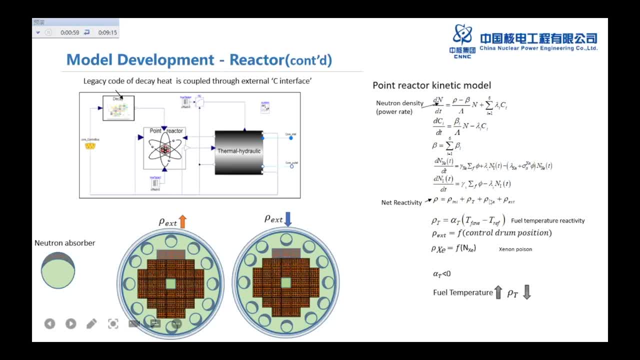 temperature reactivity and the poison, the signal, uh reactivity and also the, the, the external reactivity, which which one this external reactivity is uh, can be changed by the control drone, can be tuned by the control drum. here is the control control, control, control drum. one side of control drama is the neutral absorber. 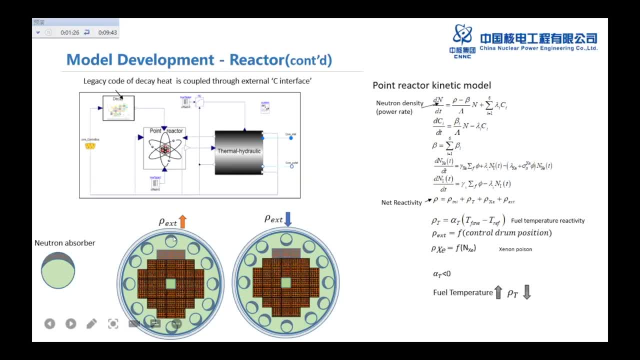 If the neutron absorber is far away from the core, then less neutron was absorbed, so the reactivity increased. But if the neutron absorber face near the react field, more neutron will be absorbed, so it decreased. And by changing the angle of this, by rotating it, we can change this term. 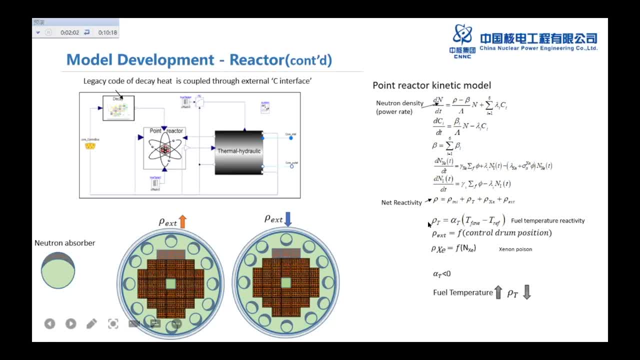 And also another important issue is that the field temperature reactivity is a function of the field temperature And because this coefficient is negative, so it gives a very good safety feature. If the field temperature rise, then this term decrease, So it's a safety feature. 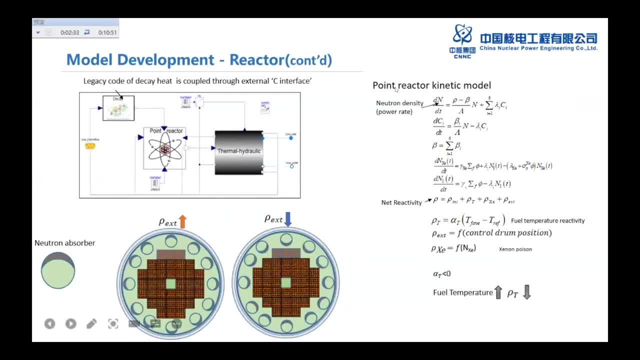 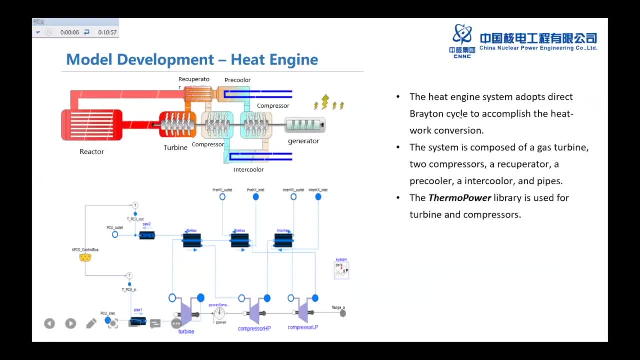 And then this is about the physics, And then the model about the heat engine, The heat engine system. we use direct helium for the Brayton cycle. And then the model about the heat engine. And this is the thermo-composed gas combined to two compressors. 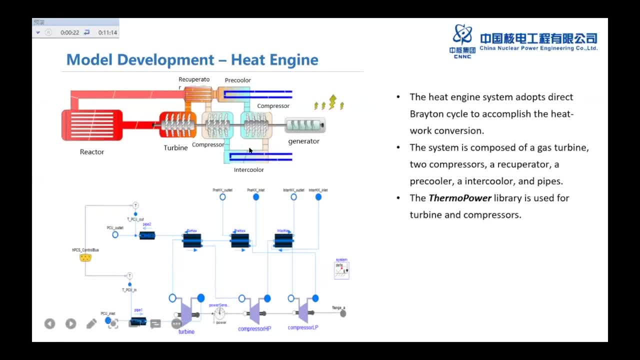 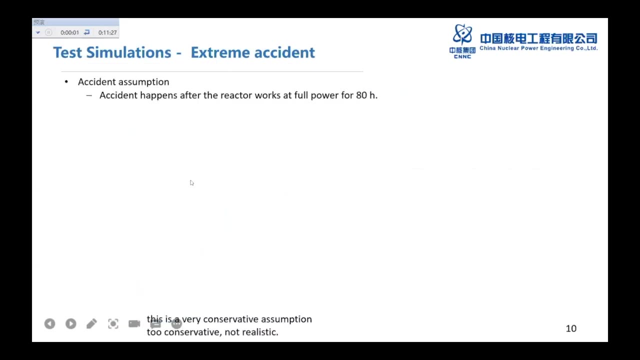 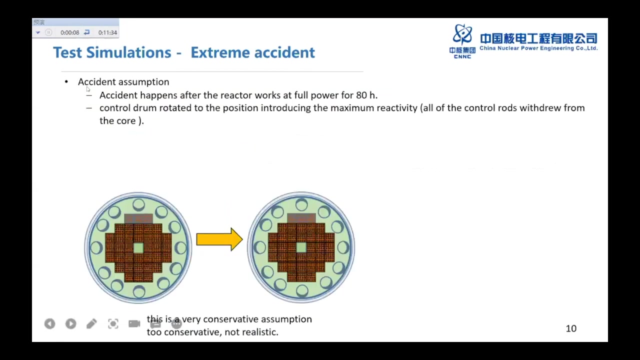 And the heat exchangers, such as intercooler, free cooler and recuperators, And in this modeling we use the thermal power library used in this model. Now I want to. I will give an introduction about the test simulation. First is the accident. 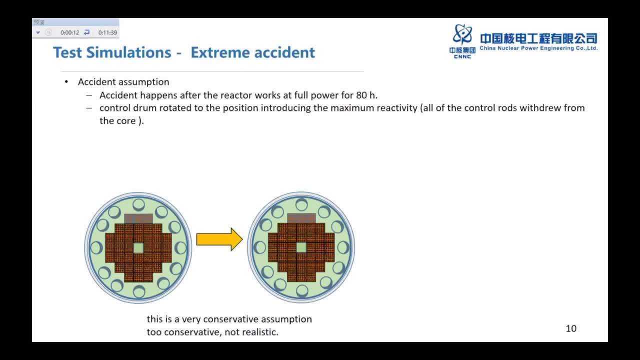 extreme accident. This accident, the assumption is that it happens after the reactor works at full power for 18 hours And at this time we assume that all the control drum rotated to the most dangerous position, introducing the maximum reactivity, Or, you can think, all the control. 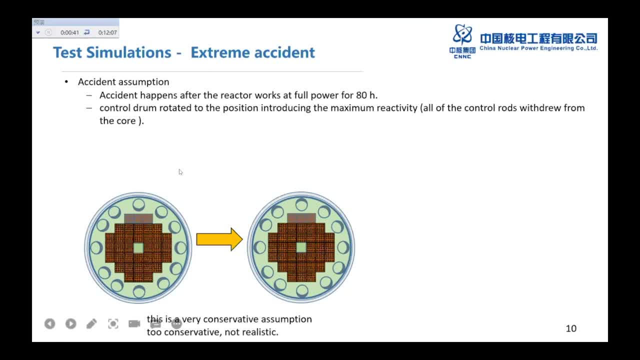 like all the control rods, withdraw from the core. It should be mentioned that this is very conservative assumption, not realistic, just of a test calculation. And also at this time the heat engine shut down and the helium flow rate drops to zero. 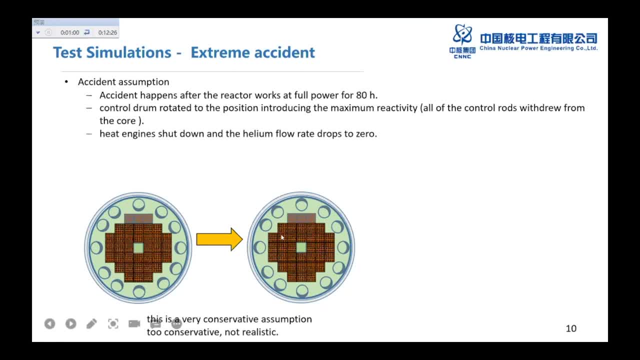 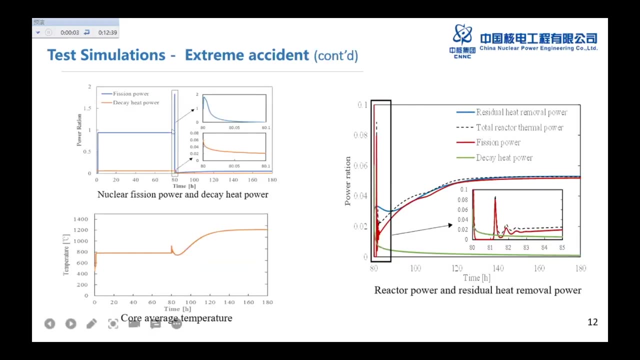 It means that the nuclear, the heat generated in the core, cannot be removed by the helium coolant flow. The simulation result is here. You can see as the control rod withdraw because the reactivity sharply increased, So the power rate sharply dropped up. 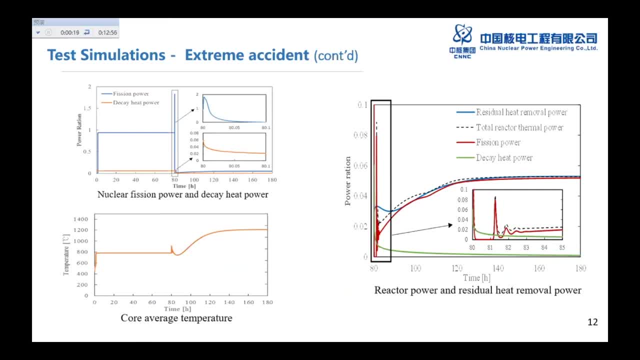 About 1.8 times of the full power And then caused the fuel temperature rise very rapidly. Because the temperature rise, because the temperature raise, and then it will give the negative feedback of the reactivity And then the fission reactor fission stopped. 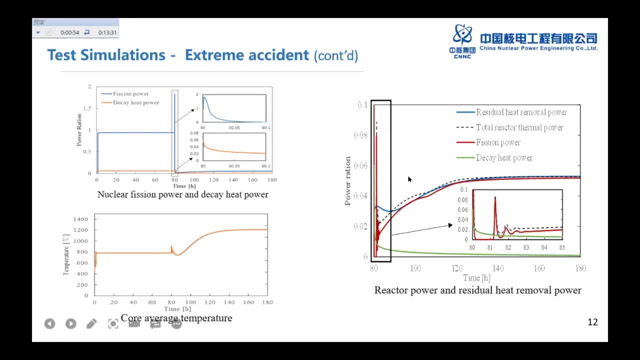 become zero And then this time, because of the heat generated in the core, still can be removed by the air cooling outside the reactor pressure vessel. So this as illustrated in this graph, So the reactor temperature decrease again, And then at some time, 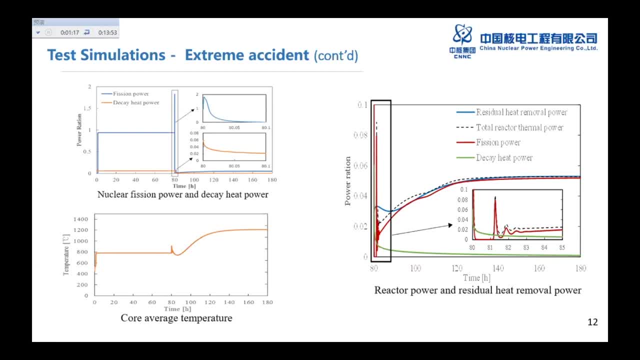 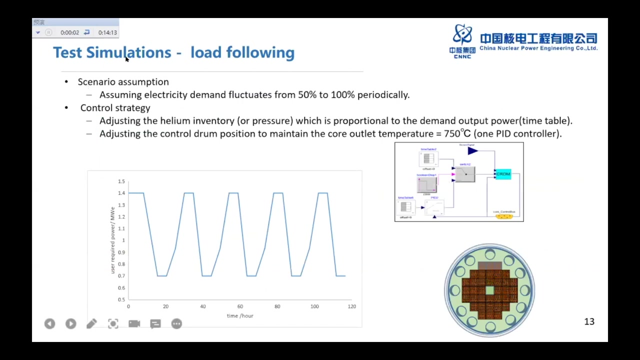 it went critical again And then finally, it achieved a stable. the stable achieved And the residue heat removed by the air cooling is equal to the total power generated in the core. This is the first one, And then it's a load falling case. 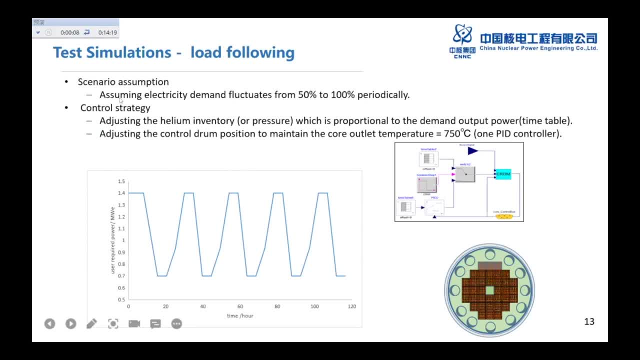 We assume the electricity demand fluctuates from 50% to 100%, And oh, I will be fast, Okay, Okay. And the control strategy is by using by adjusting helium pressure, by using a timetable. Another method is by using a PID controller. 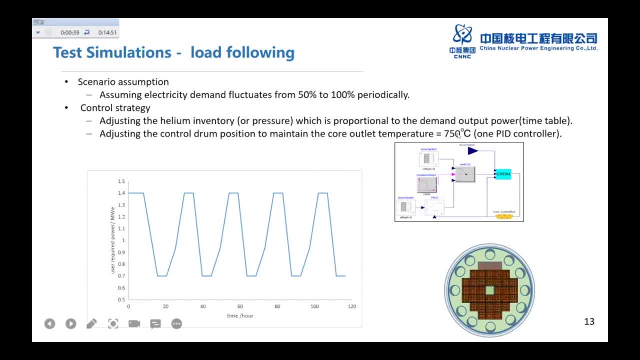 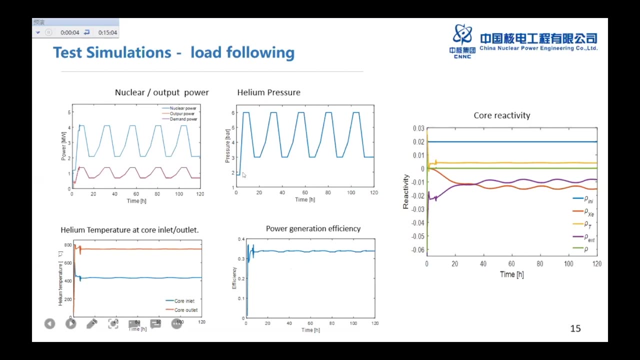 to keep the core outlet temperature at this fixed temperature and changing the drum position. And here is the result. You can see this. this output power is almost, is quite quite, the same as the demand power in this feature, And we just change the helium pressure. 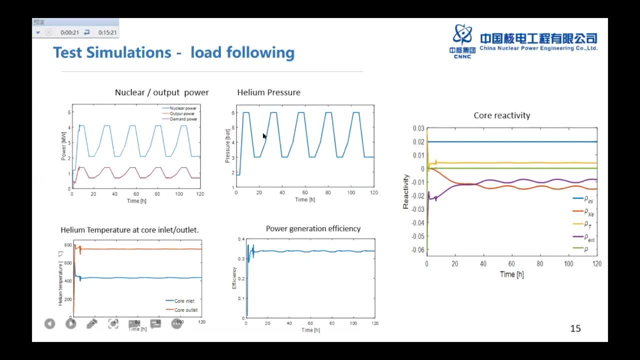